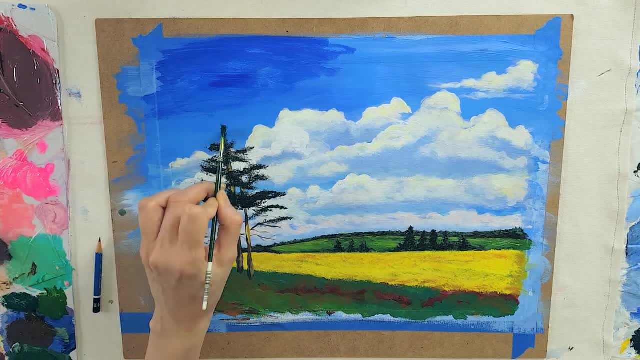 not very good for your canvas. you can use a brush that's not very good for your canvas. It's very effective in rendering foliage on a landscape, trees, even grass, And, just like dry brushing, it's more effective with a firmer bristle. 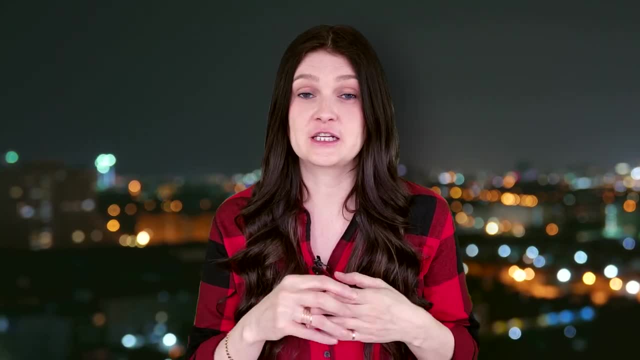 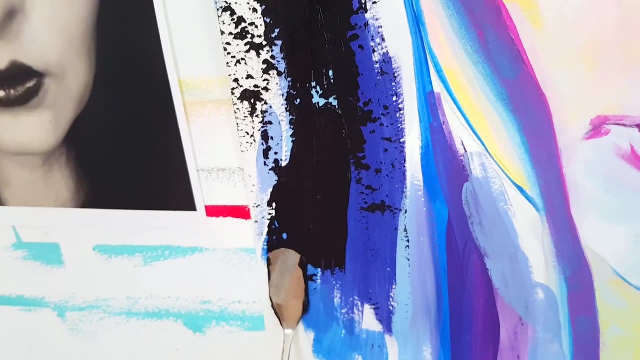 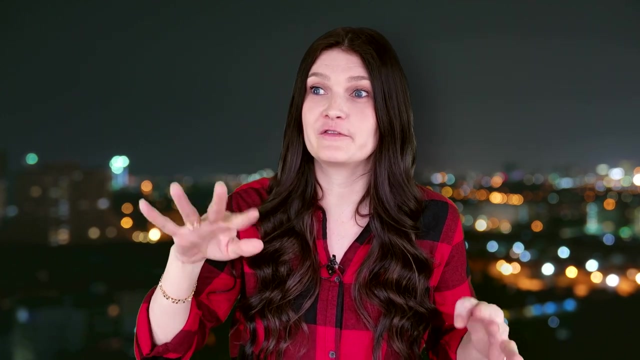 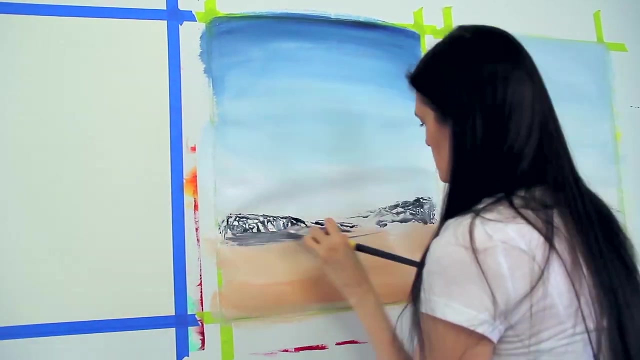 Impasto. Impasto is the action of overlapping really thick layer of paint on your canvas to create that 3D effect of texture. It can be done with a brush, with your fingers, using gloves. Some painters are finger painters, But most often impasto is used with a palette knife And you could get really realistic. 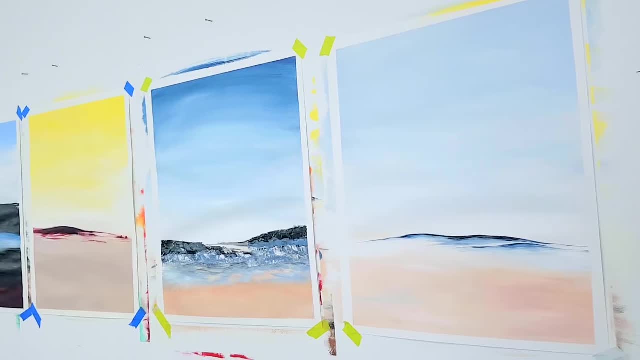 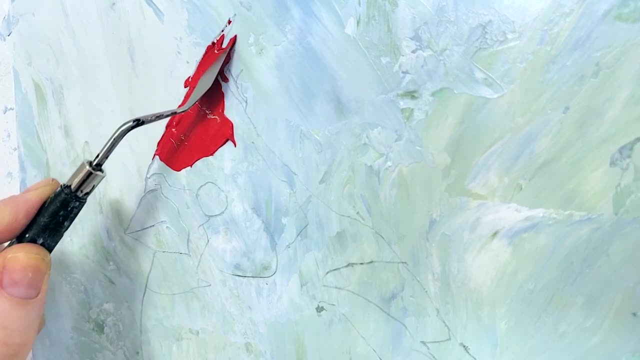 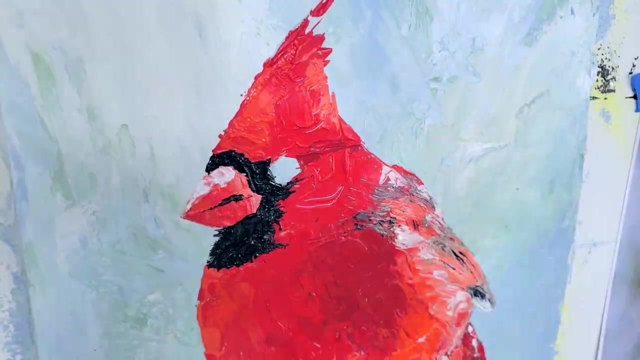 mountain tops and like a mountain range. with a palette knife, the way Bob Ross uses it, It's pretty impressive. Impasto is one of my favorite techniques, and using a palette knife can give really bold and expressive effect, especially if it's focused on one. 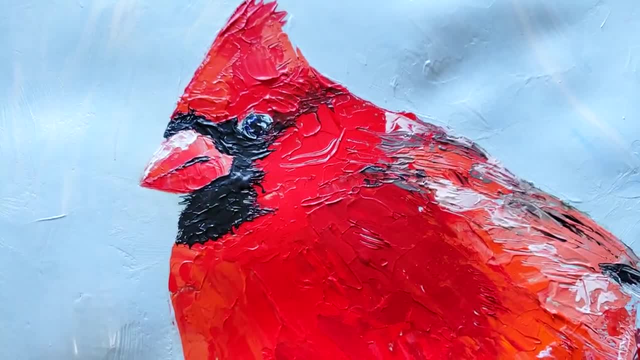 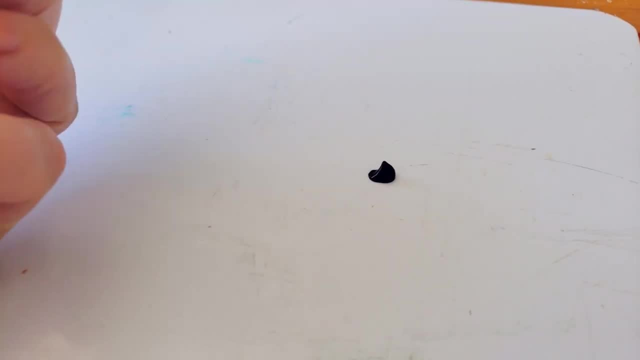 area of the painting and having the rest be with a paintbrush. It's super effective and very beautiful. Glazing- Glazing is when you apply very thin and transparent layer of paint and you layer it on top of an existing color, And the way to do it is: put just a small amount of paint. 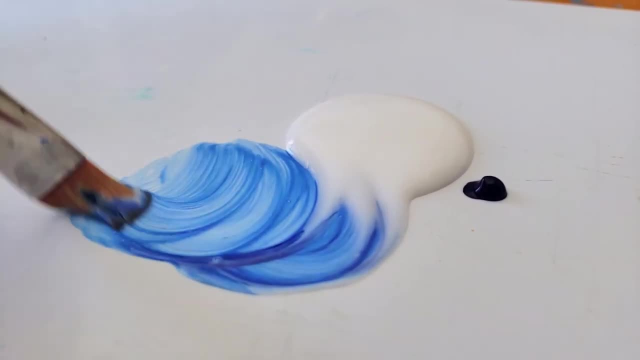 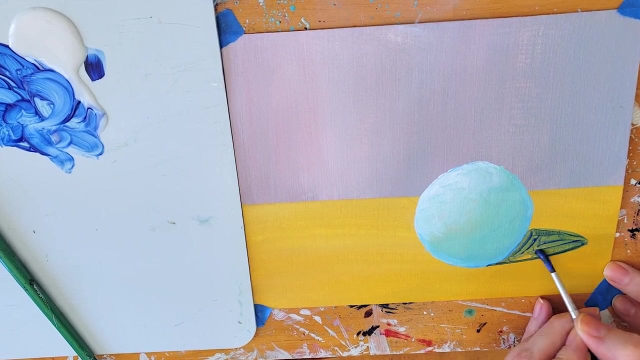 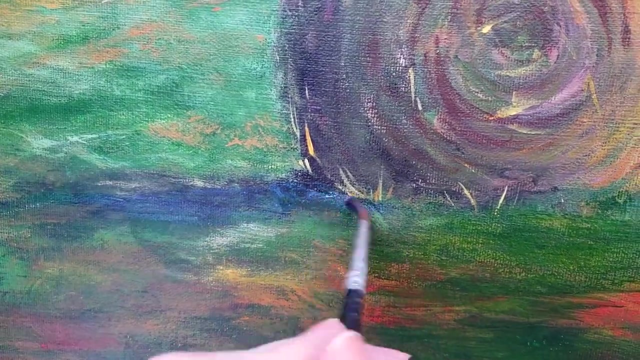 in matte medium to create a mix that is transparent, And it's used most often to create and paint shadows so that you see the underpainting with a shadow on top. It gives like a really rich and belief. It's also used to mimic some types of delicate fabrics. 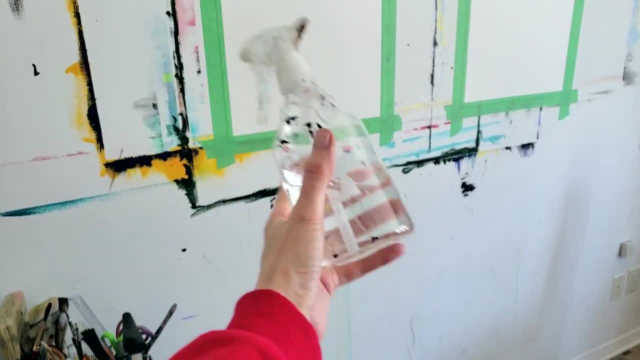 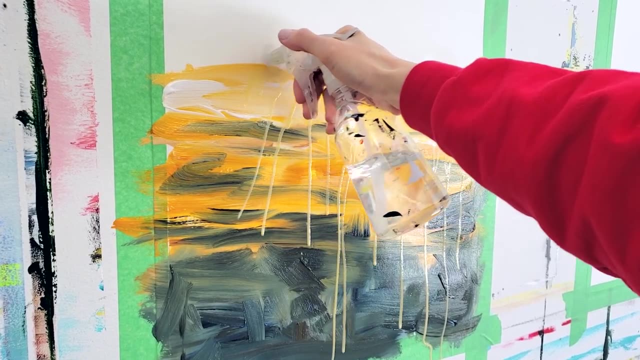 Dripping. Dripping is a wild one. It's when you spray a bunch of water on your canvas and you let the paint drip and kind of wash out and create streaks. It's used in abstract work, obviously, but it could be very interesting to use it in expressive paintings that are 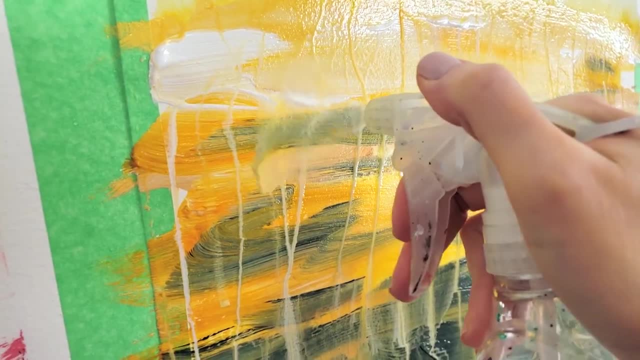 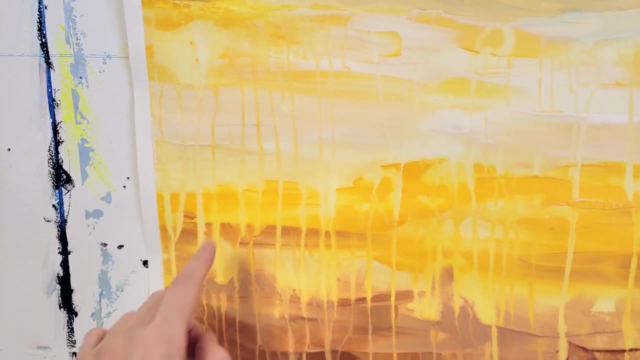 halfway between figurative and abstract. The streaks can be super bold if you use a lot of water and you leave it like that, but it could be subtle as well if you wipe sections of it with a rag and you kind of fade it within the painting. 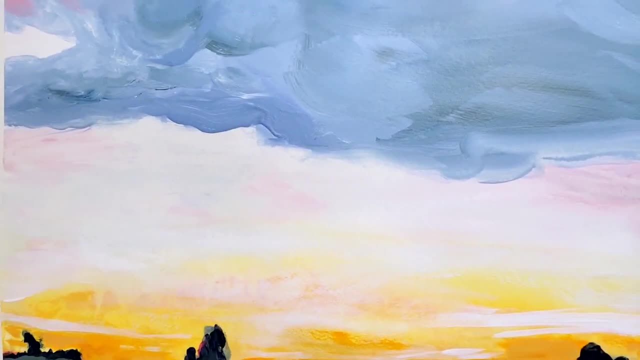 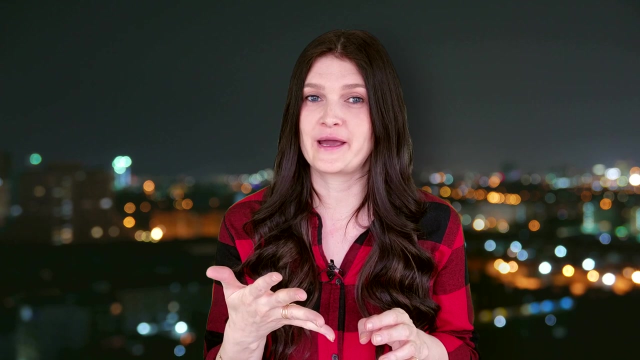 It's not for everyone, but I really love it And when it's used sparingly, it can be very effective to create a focal point in a painting. Lifting- This is another favorite of mine. It's also used with water, but in a different. 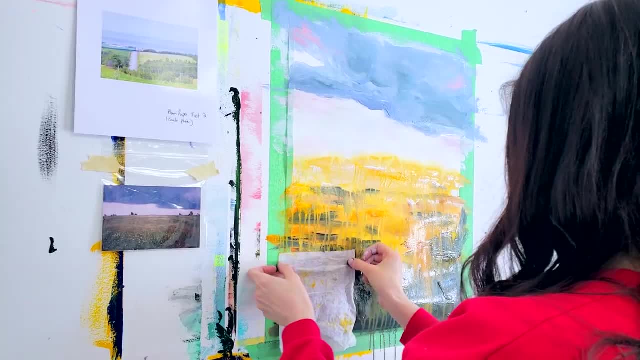 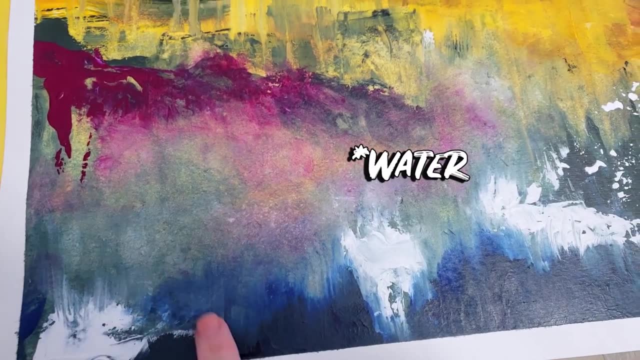 way than dripping. The key here is to have, let's say, your background halfway dried- So not fully wet, not fully dry, So not fully wet, not fully dry- And to spray some paint where you create a bunch of droplets on your canvas. Then, with 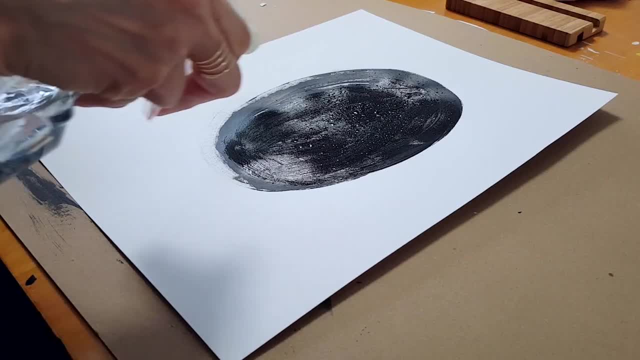 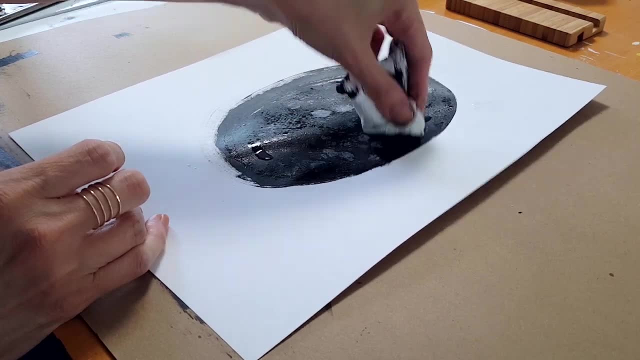 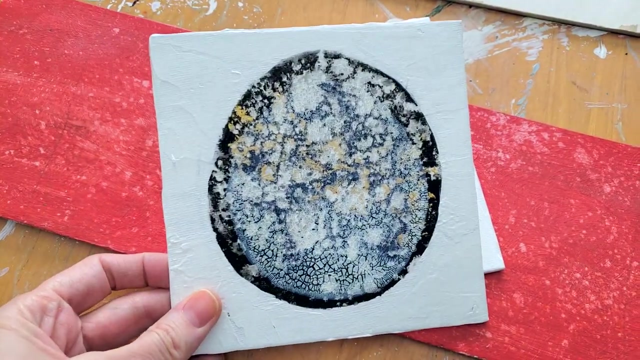 a rag or paper towel. you blot it and some of the paint will lift, creating this really beautiful, unique texture. I love it in abstract work, but it could also be a really nice backdrop for a portrait, let's say, or even to mimic snow, rain, a galaxy, anything you can think. 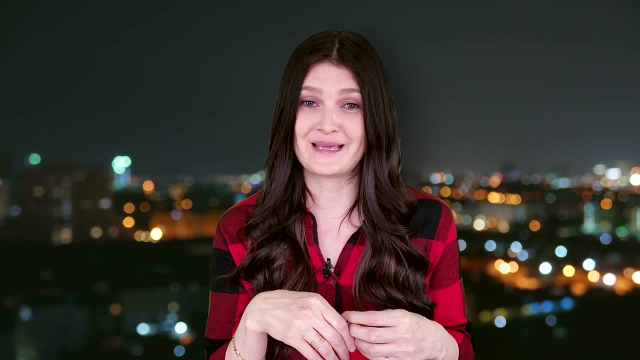 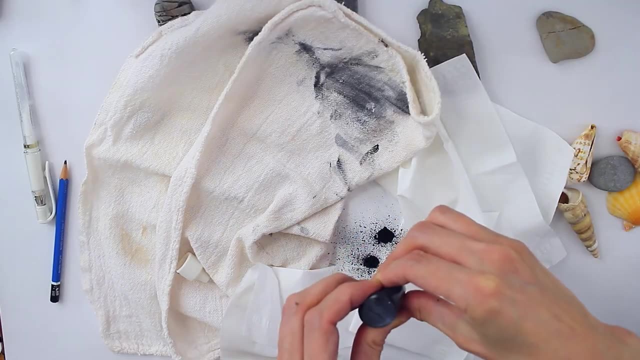 of Spattering Another wild one. It's basically flicking, like a mad person, some paint on the canvas. Obviously it's used in abstract work. It creates a lot of movement, but again it can be used sparingly in a more subtle way, The way I 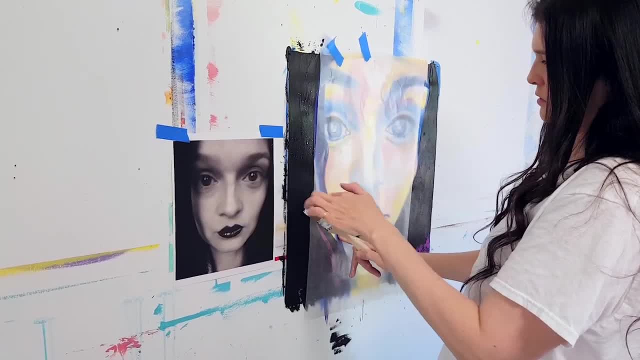 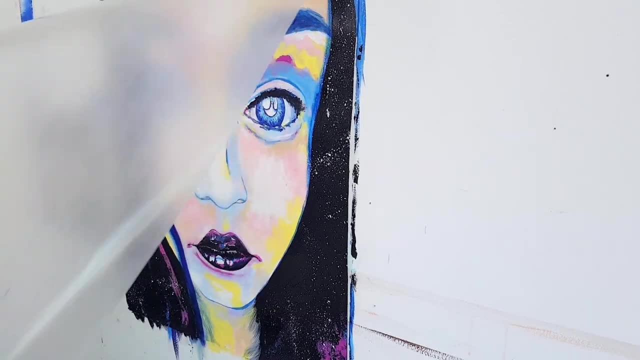 like to use it is to take a toothbrush- an old toothbrush- and flick some diluted paint on my canvas, very often to create snow. I think it's one of the best ways to use that technique- snow and a starry night as well. 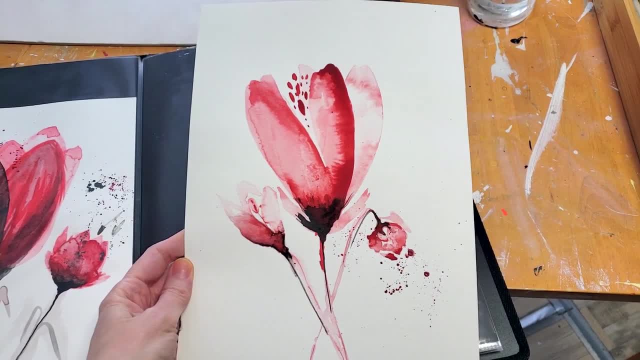 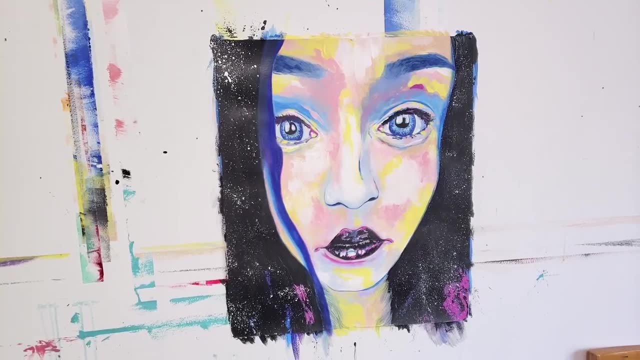 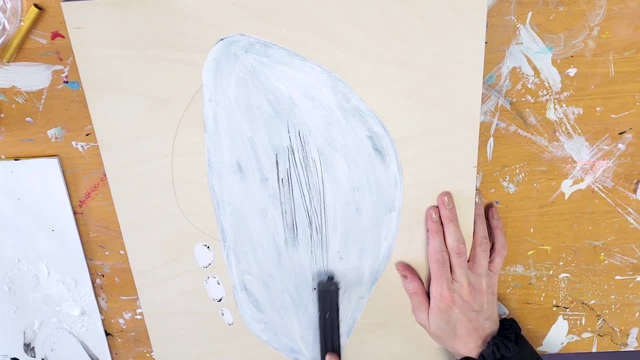 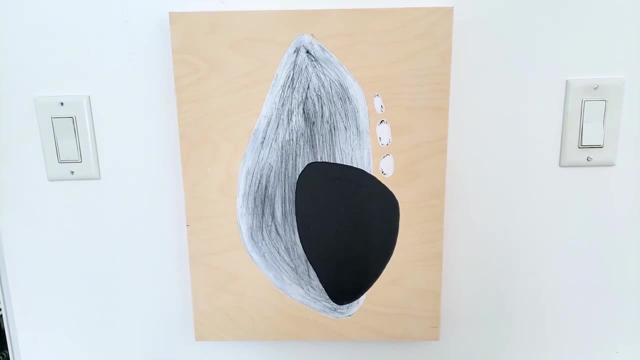 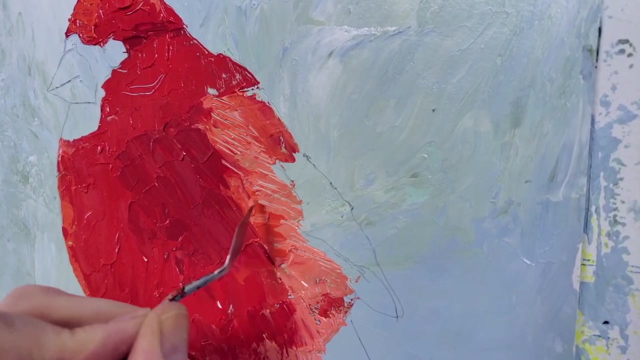 it's a really fun one to experiment with Scraffito. That's the action of scraping away some pigment on canvas, ideally before the paint dries, to create different textures. Most often it's very useful in creating hair or fur for animals or feathers. 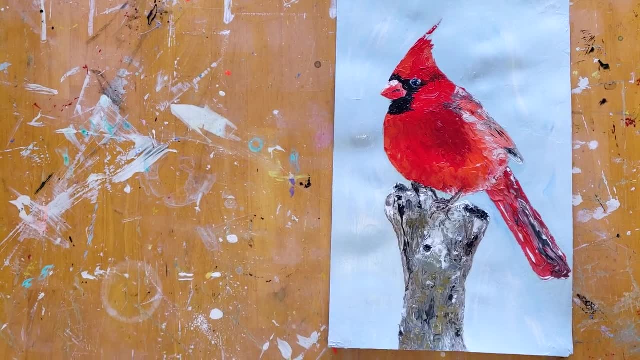 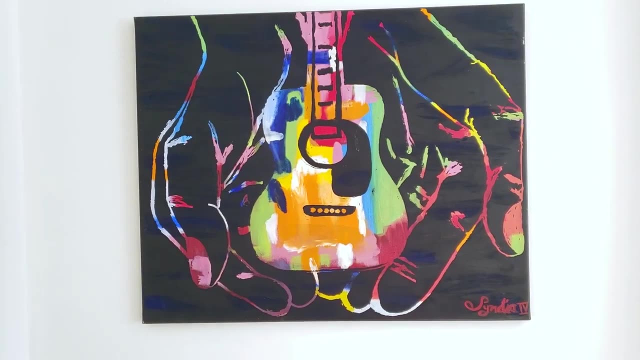 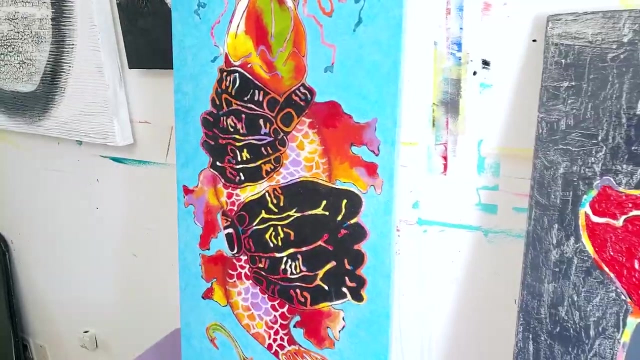 Scraffito, You can also use that technique to sign your name. I do that a lot. Masking Usually with acrylic paint. masking is used with abstract art as opposed to watercolor, where masking is used to keep the whites intact on the paper. 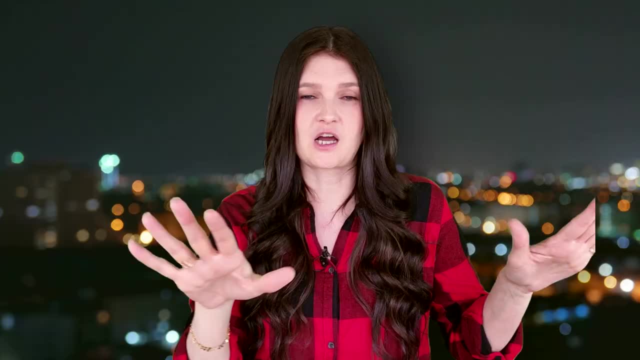 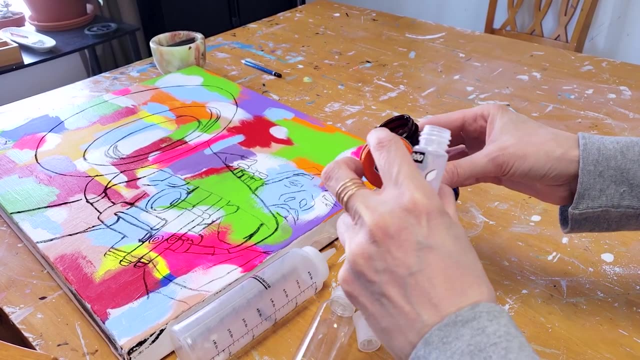 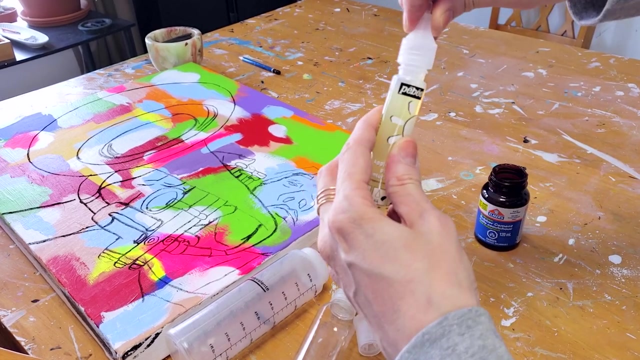 Very often masking tape is used to block off certain areas and create big blocks of colors. Obviously, masking tape can be limiting because it creates straight lines but not so much curvy lines, And that's why I like to use rubber cement. Rubber cement is kind of like a goopy glue.